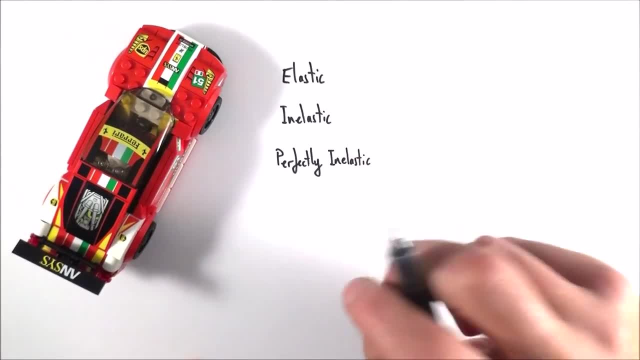 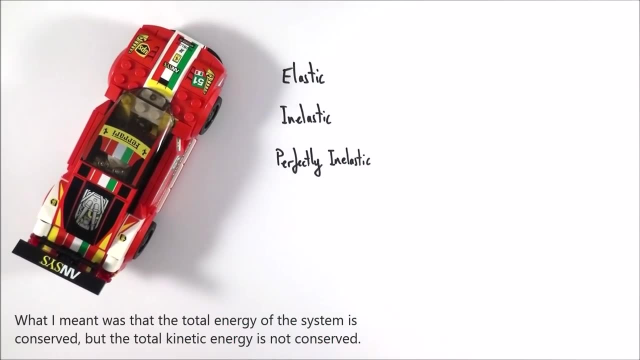 external forces apply, So the principle of conservation of momentum still applies. What doesn't apply is the conservation of the energy that those things have. For example, if you have, maybe, a tennis ball which you drop every time it bounces- it never quite bounces up to its 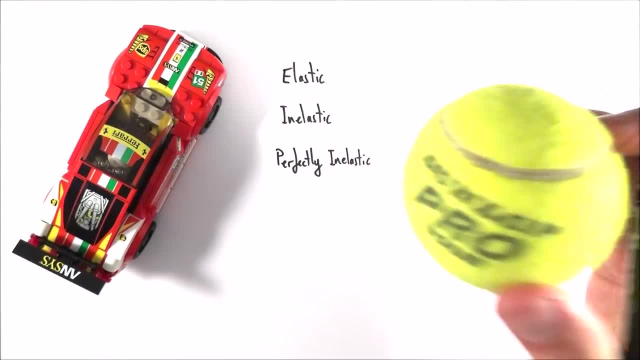 original height And what you might hear, there is some of the kinetic energy that this happens to have. So if you have a tennis ball which you drop every time it bounces, it never goes as fast And that's what we've had initially being lost as sound energy, and there will be some. 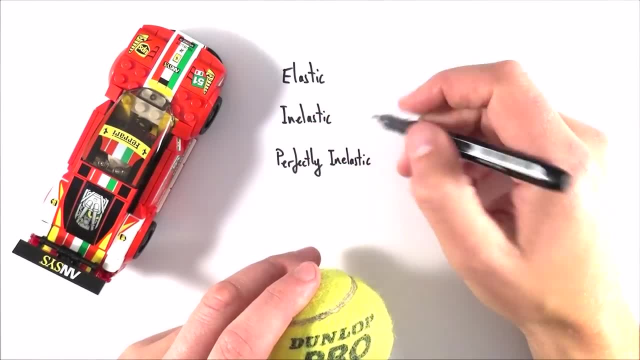 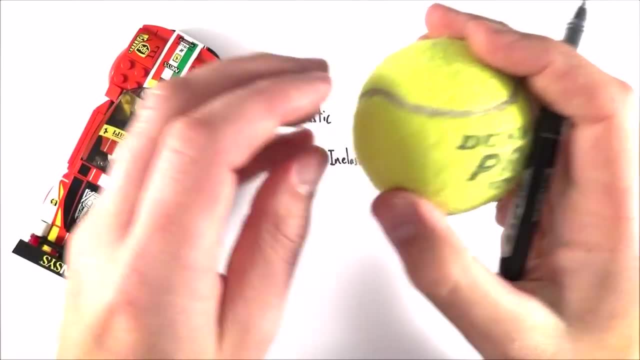 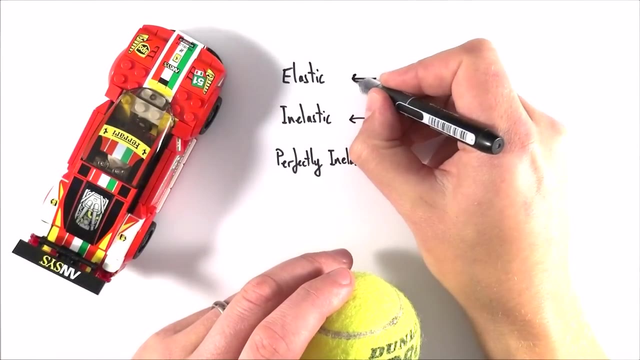 heat energy as well. So in an inelastic collision what we have is that kinetic energy is lost from that system. So two things might collide, they might bounce off but not go as fast and therefore kinetic energy is lost and therefore that is an inelastic collision. Elastic collisions, this is 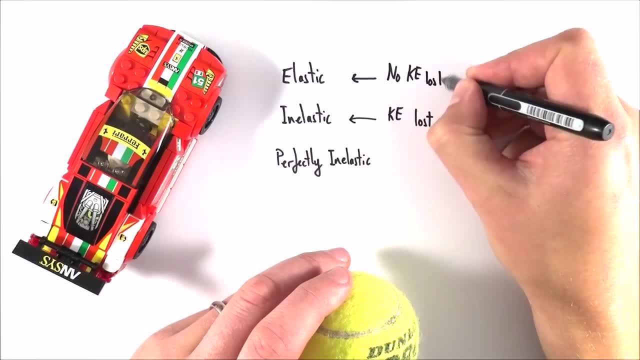 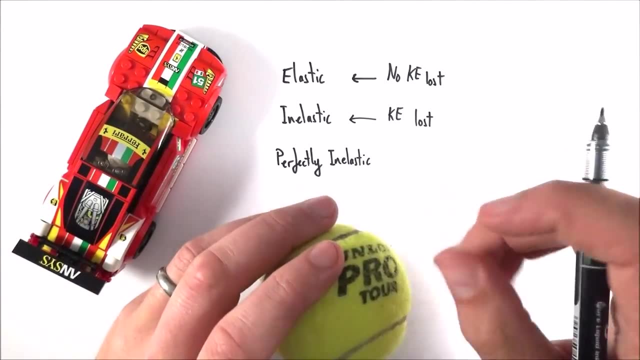 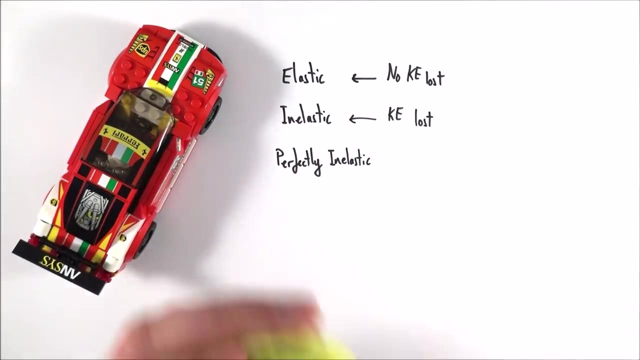 where no kinetic energy is lost, And that means whatever the total kinetic energy is before the event, we have the same kinetic energy afterwards. Doesn't really happen that much around us. but if we consider maybe the motion of particles in a gas, we can consider them to be perfectly elastic. collisions, Finally, perfectly inelastic. What? 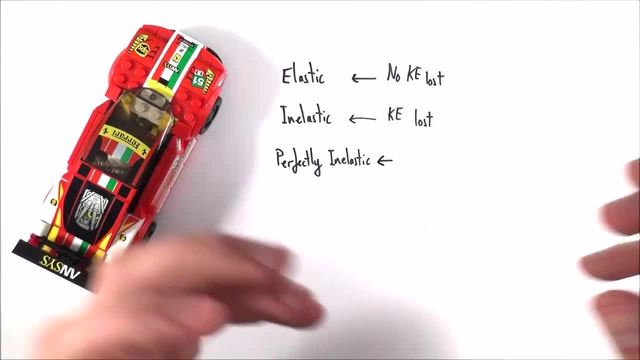 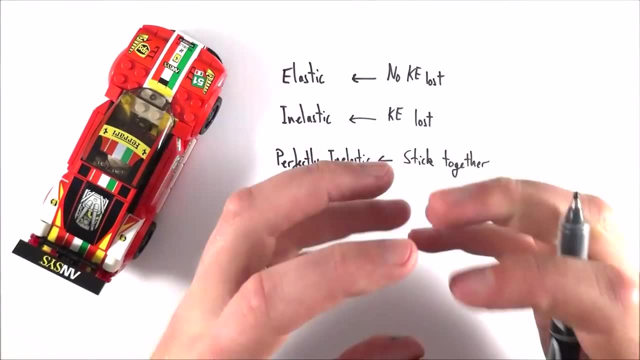 does that mean? What's the difference? Well, perfectly inelastic is when two things collide and then afterwards they stick together. For example, you might have a bullet that goes into the target and the two things stick together. And if that's the case, and the two things move. 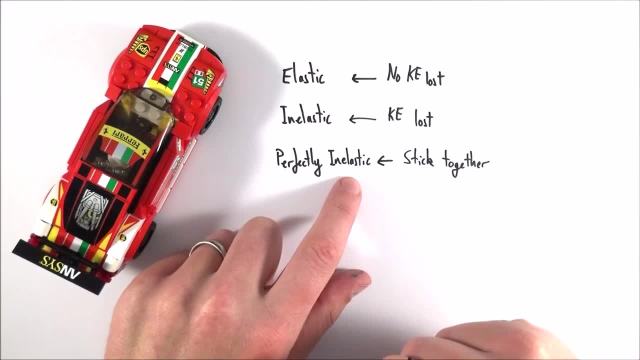 off together. afterwards we have a perfectly inelastic collision And there's a little symbol that we can use to really tell us about these collisions, and it's a symbol: little e. Now, little e. this stands for the coefficient of restitution, And we can work out e by looking at. 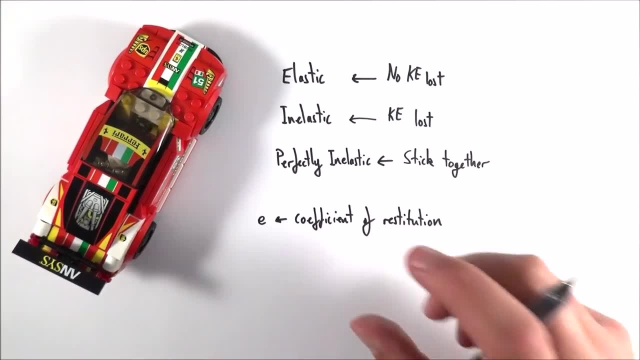 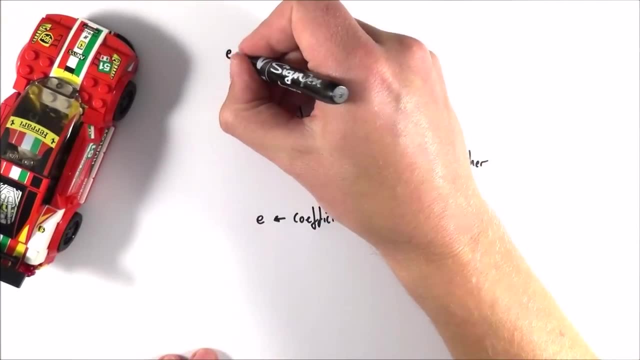 the relative velocity of the bodies before and after the collision. You don't need to know a huge amount about it, apart from to say if we look at these different collisions here and we actually look at the value of little e when we have an elastic collision, the value of little e. 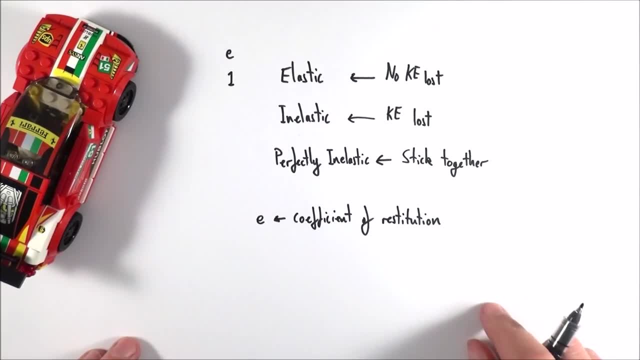 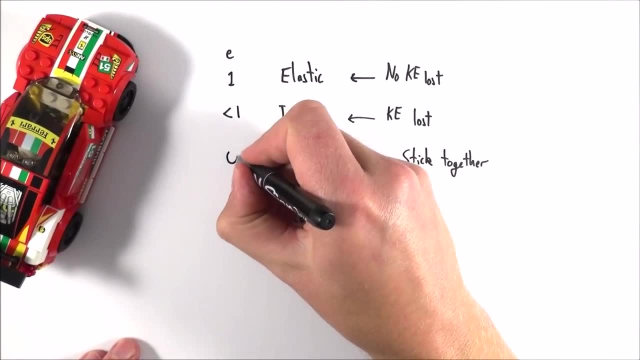 is one, So the value of little e is one. and the value of little e is one, So the value of little e is one. So the velocity of things coming in is going to be the same as the velocity of things coming out. If the value of e is less than one, we have an inelastic collision. And if e is zero, 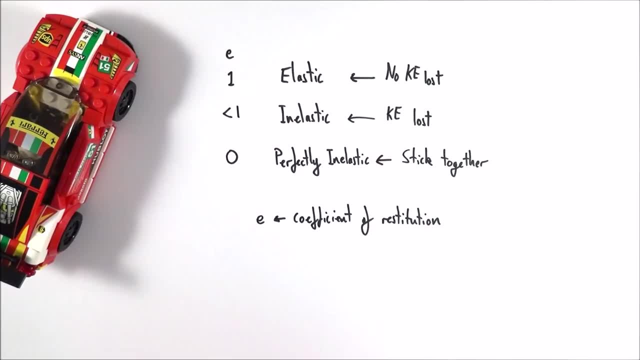 which means that things stick together afterwards. then we have a perfectly inelastic collision, And this is really that defining equation which gives us the value of e. It's the relationship between how quickly things move apart after they've been moving towards each other. The smaller, the